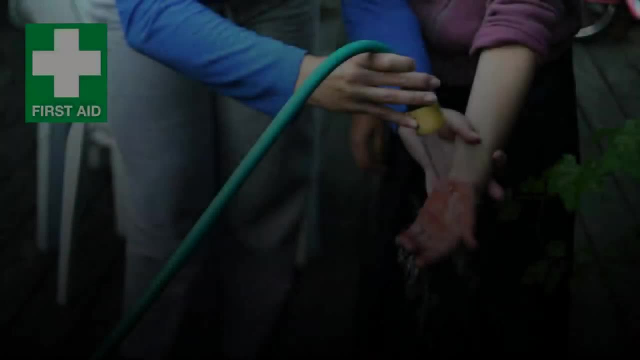 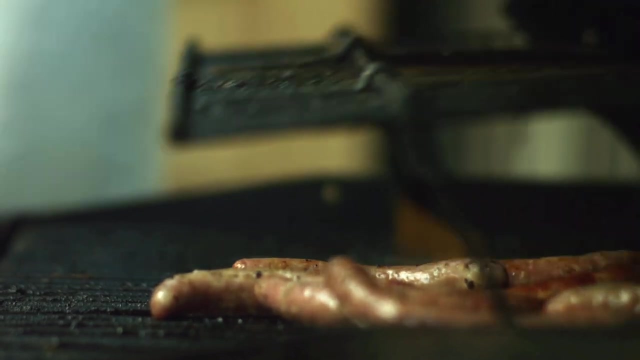 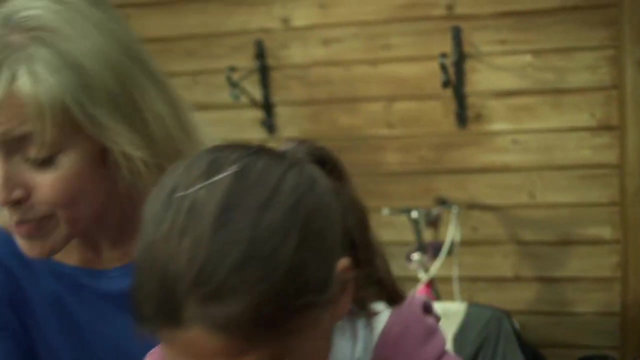 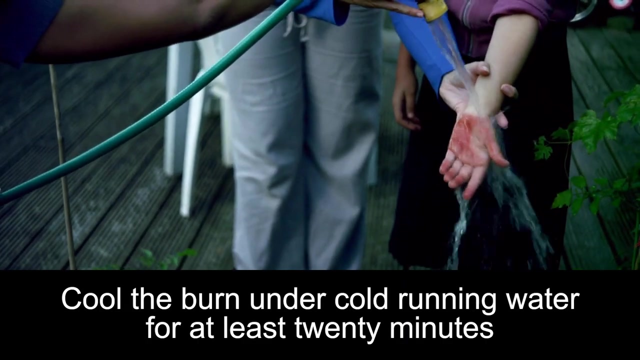 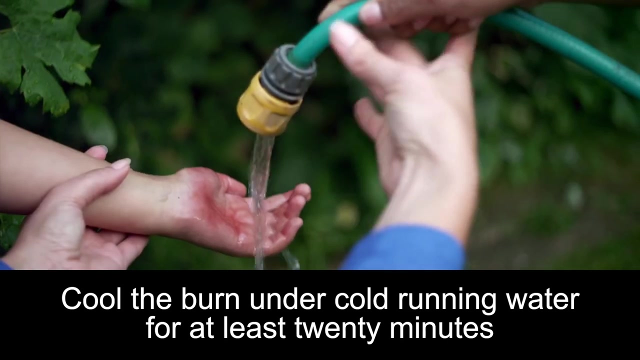 First aid for burns. Ow Sarah, can you get some water please? The hose, We're just going to put some cold water on it and soothe it. Cool the burn under cold running water for at least 20 minutes. Does that feel better? 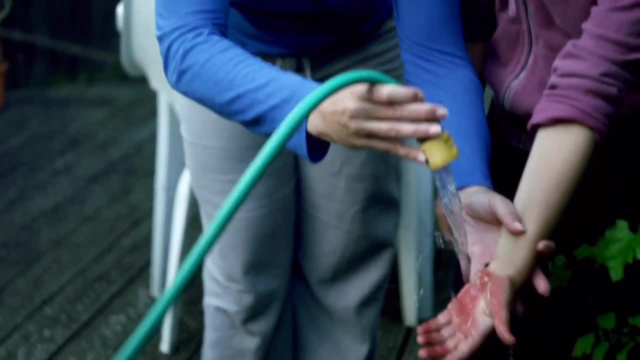 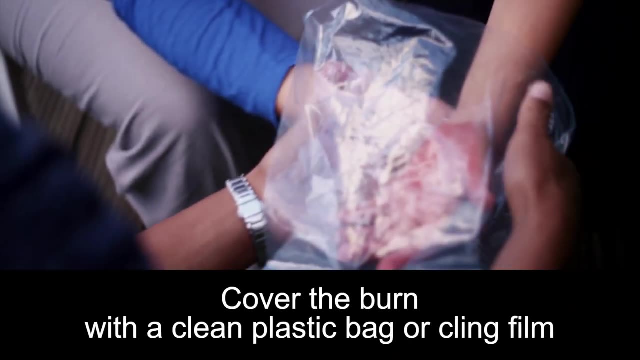 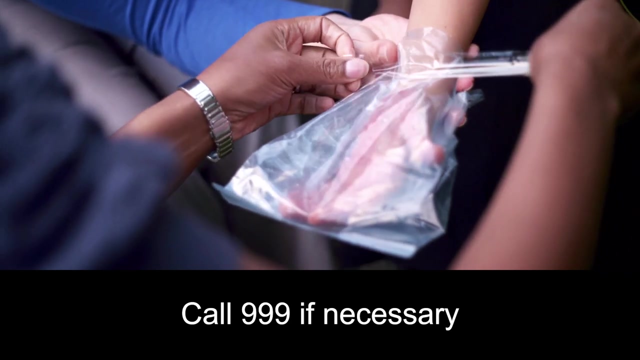 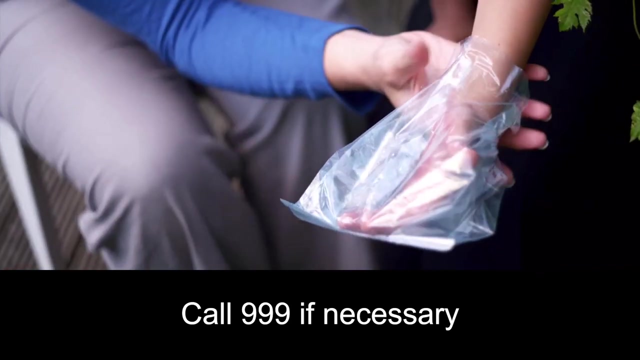 Get me a freezer bag and some tape as well. please Cover the burn with a clean plastic bag or cling film. This will keep it clean and it won't hurt as much. Call 999 if necessary. That's it. I think we need to go to hospital.